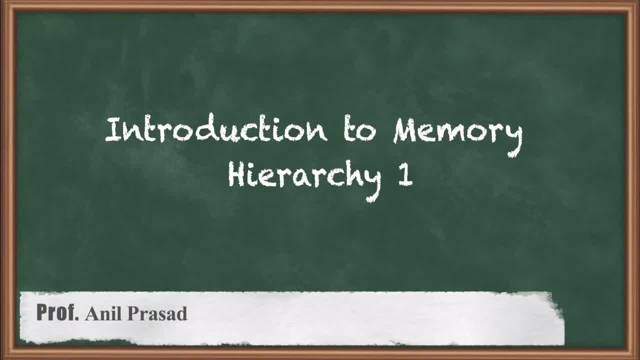 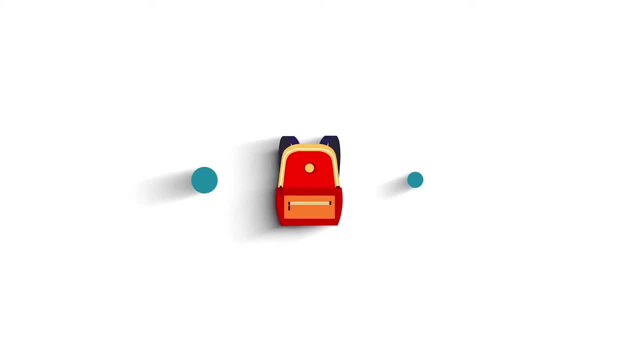 In this session we are going to start and look into a new topic, which is called memory. You know that memory holds an important role, an important place in the entire computer architecture, Because you know that a program is needed to be stored in the main memory. 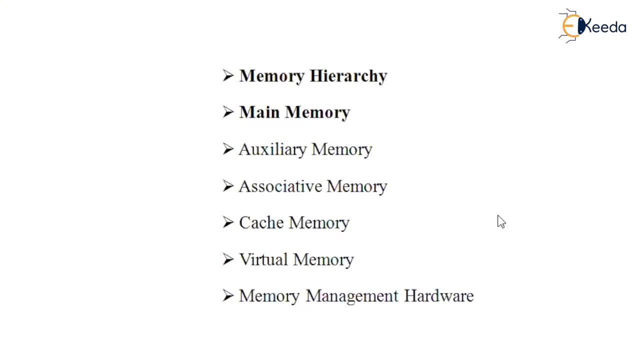 that is the physical memory before it gets executed. That is the fundamental rule of a program: to execute. You know that everything is a program in the computer system. That is, either you move a mouse or watch a video, or you play a game or you listen to a song. 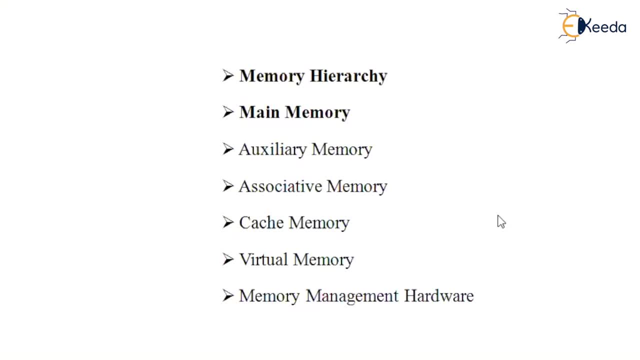 anything will eventually get converted to a program And finally, when the program gets executed, you are going to get the desired output. Now you need to understand how important is the main memory, Rather, how important is the memory, Because not only the main memory, we do also have something called secondary memory. 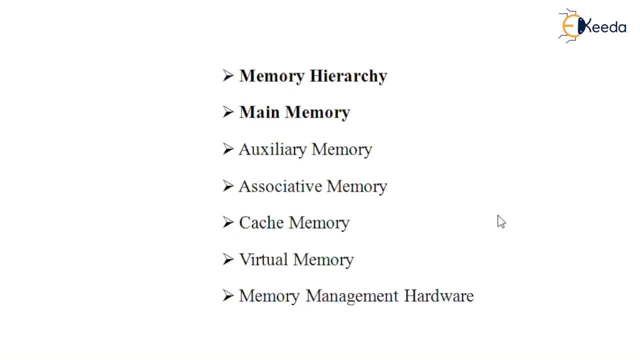 Now, in this topic of memory, we are going to completely distinguish between various memory components. Now the things are as follows: The topics that we are going to cover. the agenda is as follows: First we will discuss about the memory hierarchy And then we will talk about the main memory. 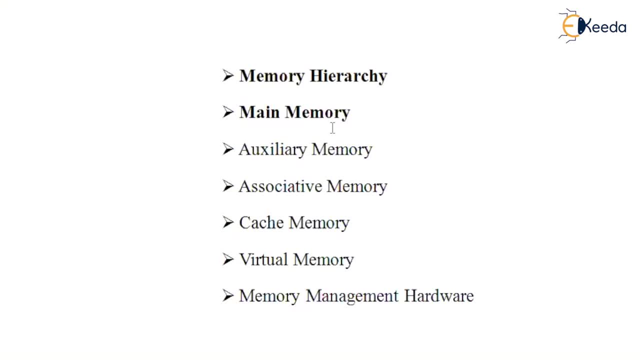 which is the important memory in the computer system And when it comes to the CPU. as far as the CPU is concerned, the only memory unit that is available is main memory, And then we will talk about some secondary memory devices, how those are going to work. 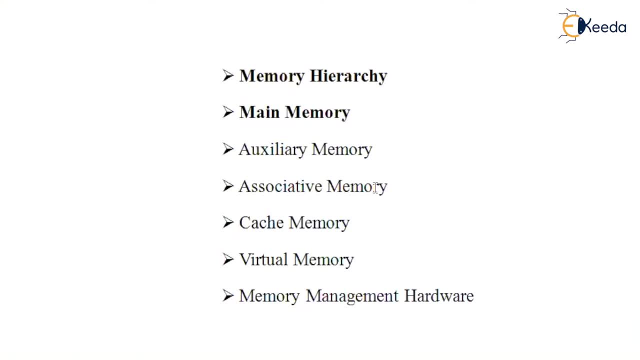 Then we are going to discuss something called associative memory And, finally, the important concept in the entire memory topic is cache memory. We are going to have a look at and we'll completely immerse into the topic of the cache memory, Because this cache memory is very important. 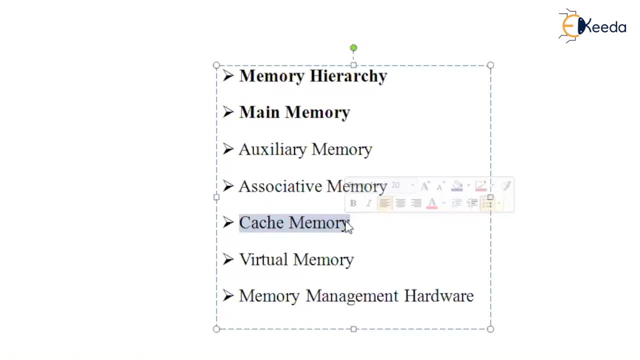 From the perspective, from the point of view of the GATE exam, most of the questions you may get from cache memory. okay. So cache memory has n number of subtopics. We are going to get into each and every subtopic and we're going to understand to the extent it is required to solve the GATE exam. okay, 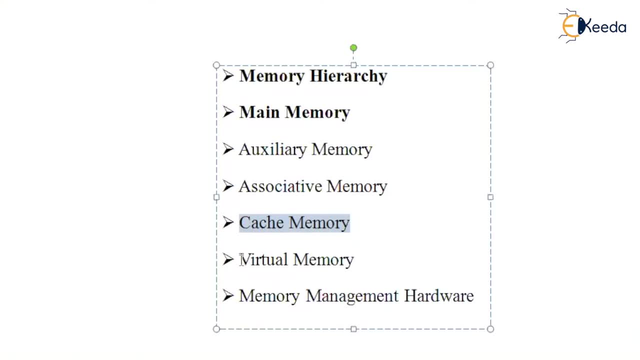 Now next is virtual memory. We understand what is virtual memory and why the virtual memory is needed. So we are going to have a look at and we'll completely immerse into the topic of the cache memory And finally we just go for a memory management system in the entire computer architecture. 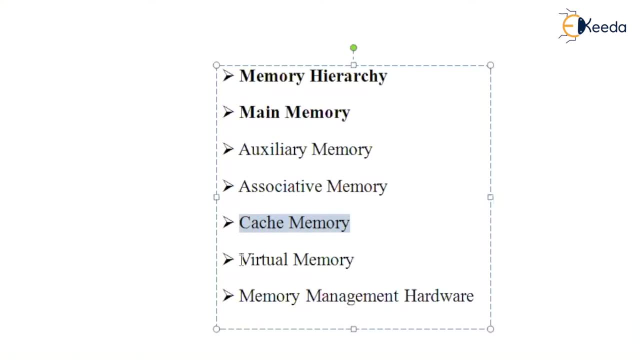 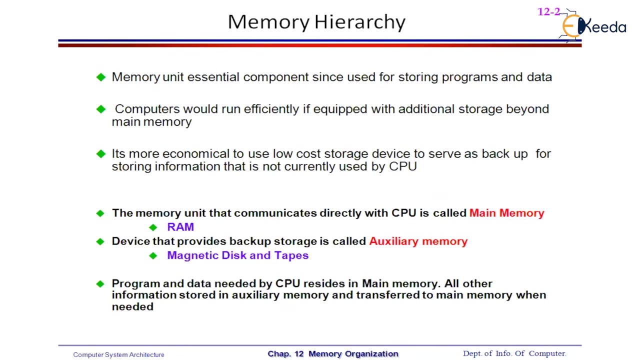 Because when memory is there, the memory is properly need to be organized. So what are the various organization techniques we are going to cover in this topic? Let us start Now. when it comes to the memory hierarchy, you know that memory unit is a very important part of the system. 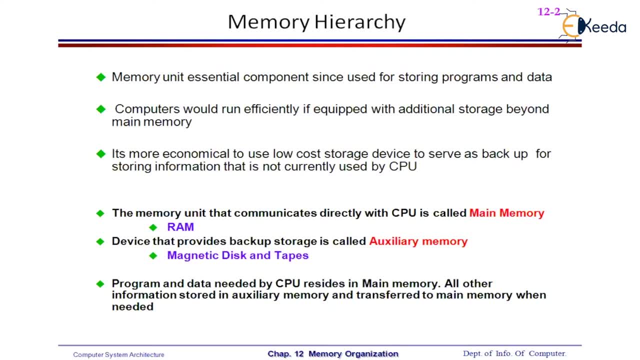 It is an essential component, since used for storing programs and the data, because you know that if you want to store the program you need to have a memory. If you want to execute a program, first of all that program is needed to be stored Where In the memory unit right. 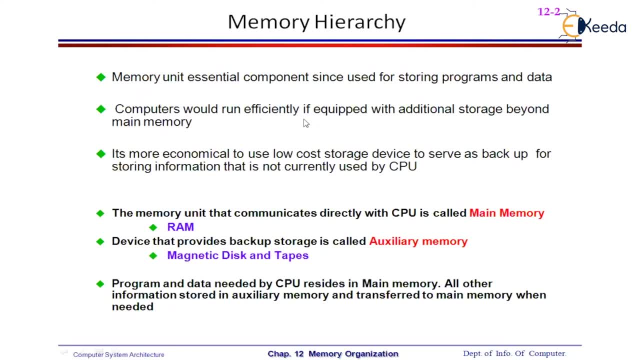 Computers would run efficiently if equipped with an additional storage beyond the main memory. When it comes to the CPU, CPU just holds main memory. Main memory is very small. When it comes to the main memory. the main memory is very small. Now, we do require some additional storage to store all the programs, all the files, everything that we do have. 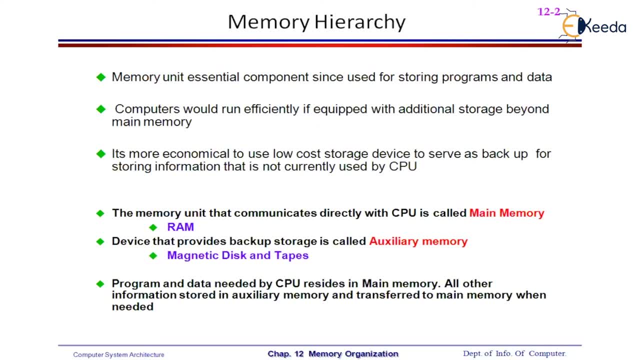 Because main memory is too small to accommodate all the programs, what we have. For an example, look at your hard disk size. The hard disk size could be 1TB to 2TB. Anything can be stored in there, But when it comes to the main memory, main memory is very small. 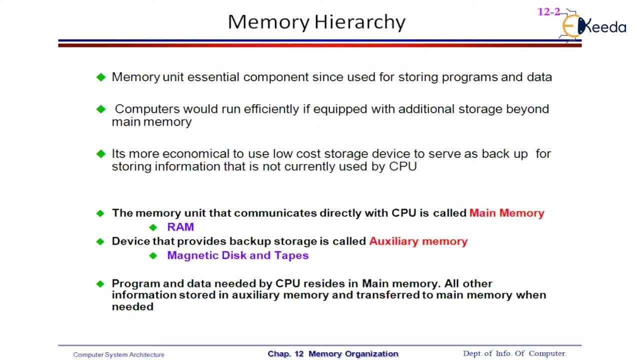 Main memory could be around 2GB to 4GB, a maximum of 8GB. So if you want to execute multiple programs, of course it is possible in the main memory. But the number of programs, the total number of programs that we have, can not be accommodated any time in the main memory. 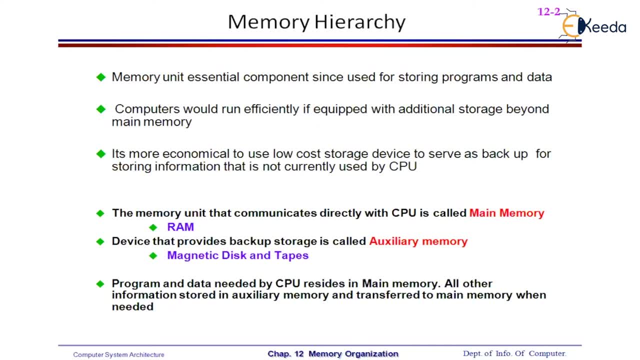 Because the total number of files- we call it as the programs- in the computer system are pretty much more than that of the size of the main memory. There is a reason why we do require an external hard drive, Some additional memory logic, to store all the files and the programs that we do have. 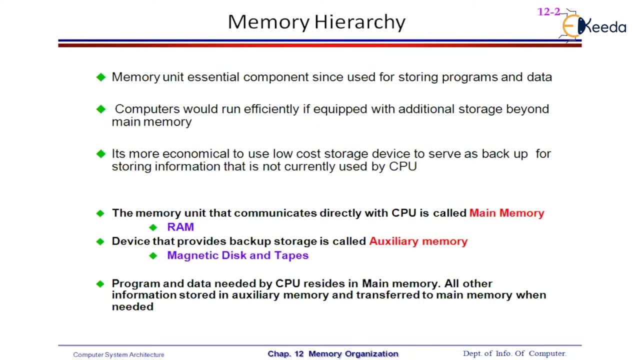 Whenever we want to execute any particular program, we will get it transferred from secondary memory to the main memory, Because this is an important rule to execute any program. Okay, next, It is more economical to use a low-cost storage device to serve as a backup for storing information. 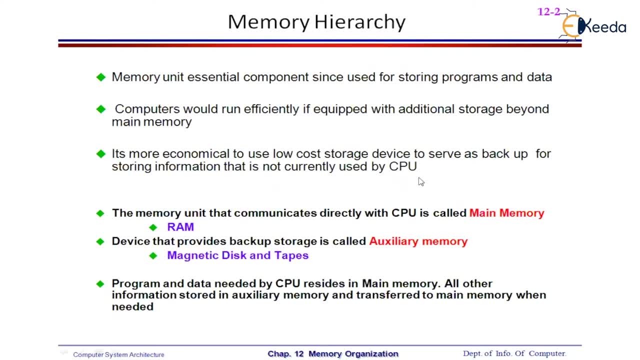 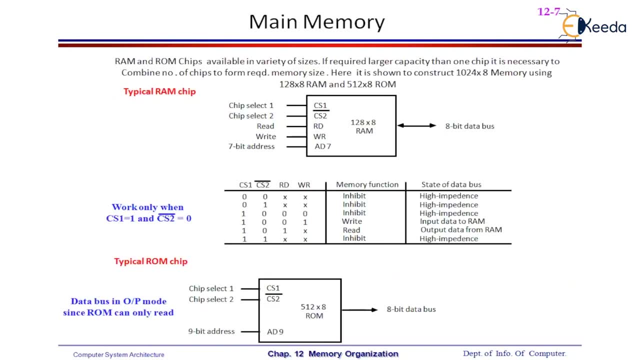 that is not stored in the main memory. So the main memory is not currently used by the CPU. What will be there in the main memory? The main memory is just going to hold. Let me show you. This is main memory. This is main memory. 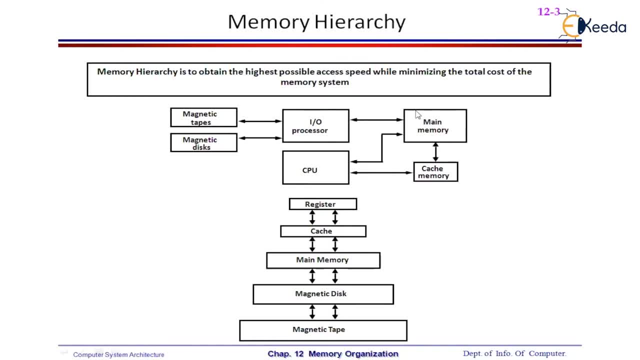 This main memory is going to hold the current programs that are getting executed by the CPU. Okay, this is the CPU. The main memory is simply going to hold the current programs, That's it. But there are many programs other than the current programs that are getting executed by the CPU. 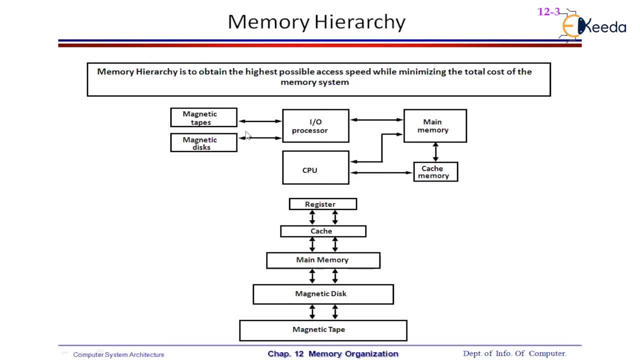 that are getting executed. for that, what i do is i will take some additional storage logic. nowadays, magnetic tapes and magnetic disks are no more used. rather, we are going to use optical disks such as hard disks. okay, so initially what i do is i will take a hard disk. in the hard disk i'm going 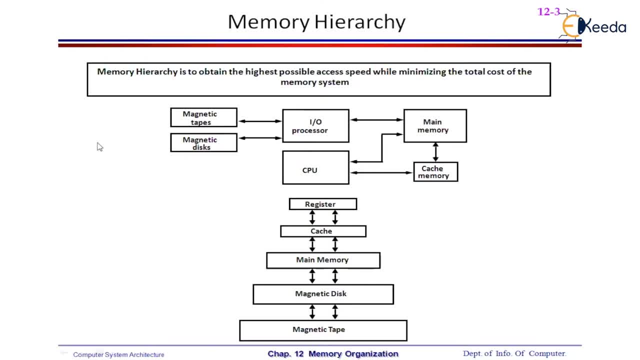 to um store all my programs whenever that program is needed to execute. that program will get transferred to the main memory and thereby from the main memory to the cpu. uh, the execution will start. cpu is going to get the programs from the main memory and they will get executed. 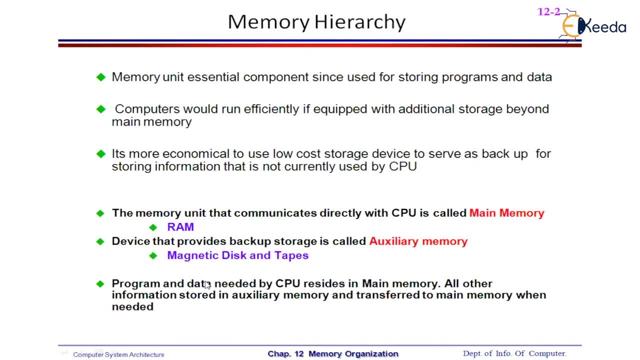 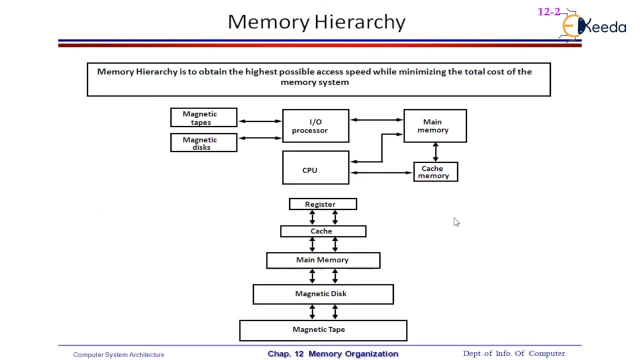 and then the memory unit communicates directly with the cpu. that is called main memory. the only memory that we do have in the system is the main memory. this main memory is directly connected to the cpu. okay, now, when you look at your malware, you will realize that when you put this data in a mobility generator, its mainly 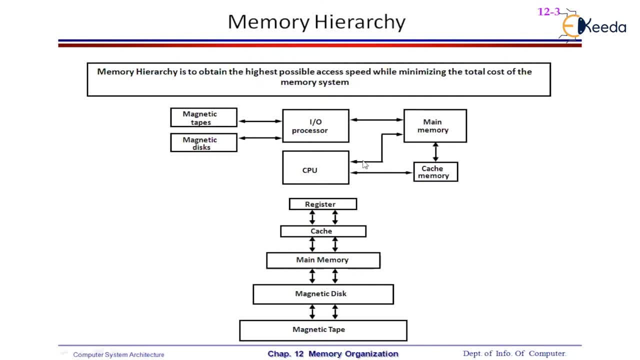 motherboard, not only in this block diagram. just open your motherboard, open your computer system, just look at your motherboard. On the motherboard itself there is a slot for the main memory and when you insert main memory into that slot, then the CPU is going to use the main memory which is available. 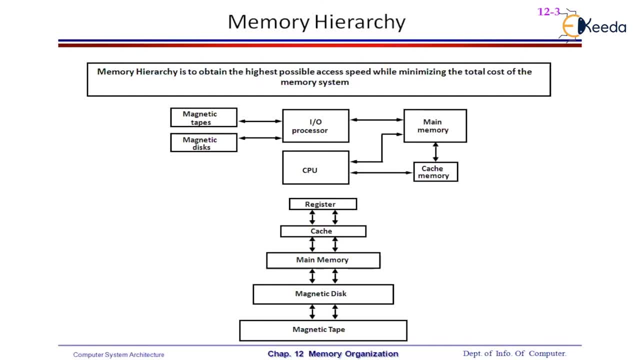 in the motherboard which is available on the motherboard. Now, the only memory for the CPU is main memory, because this main memory is directly available on the CPU motherboard. okay, So the main memory is considered to be the only memory that is available for the CPU. 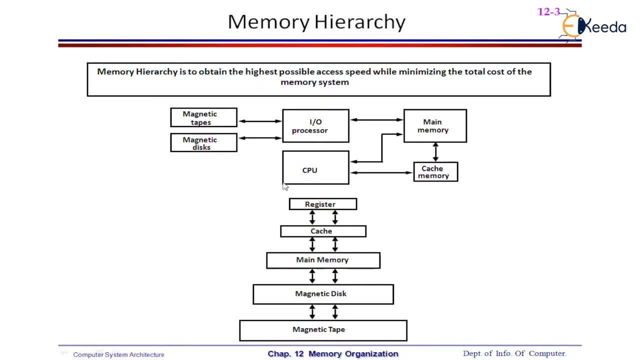 but when it comes to the secondary memory, CPU doesn't consider secondary memory as an internal part. Secondary memory is somewhere at the outside world. Secondary memory is quite similar too. Any of the peripheral devices- okay. So CPU treats all the peripheral devices such as keyboard, mouse or any other peripheral 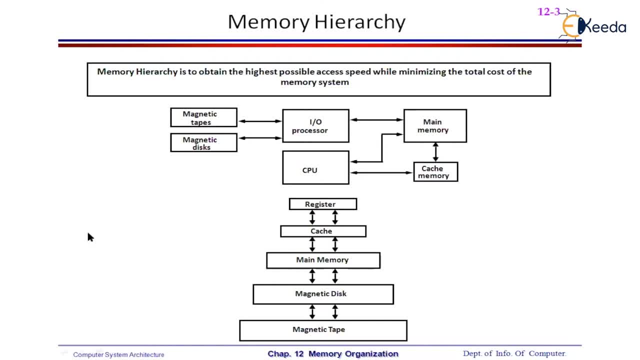 device that you have and the secondary memory, that is hard disk, same alike. CPU is going to treat all the peripheral devices and the secondary memory one and the same. okay, Now there is a cache memory. I'm going to talk about this cache memory. 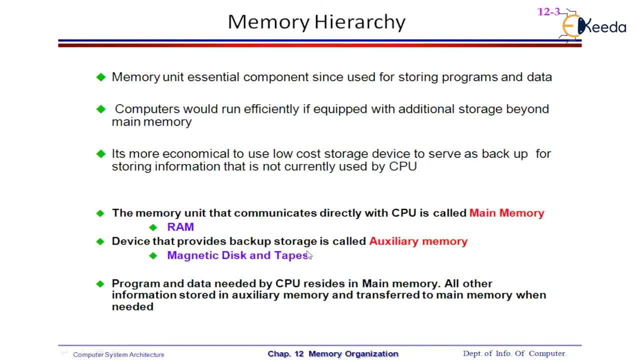 In the case of the memory in a short while. okay, The device that provides the backup storage is called auxiliary memory. Nowadays we're not going to use. we were not using this disk at all. Nowadays we are using just the hard disk. 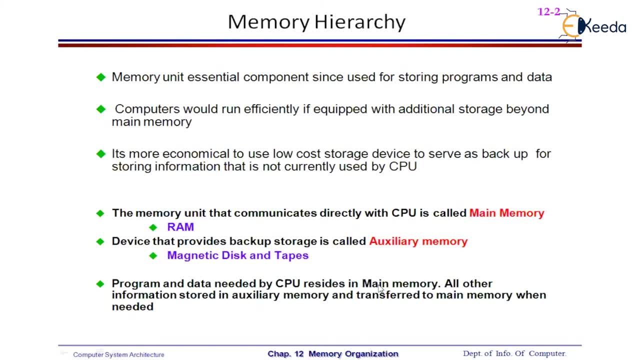 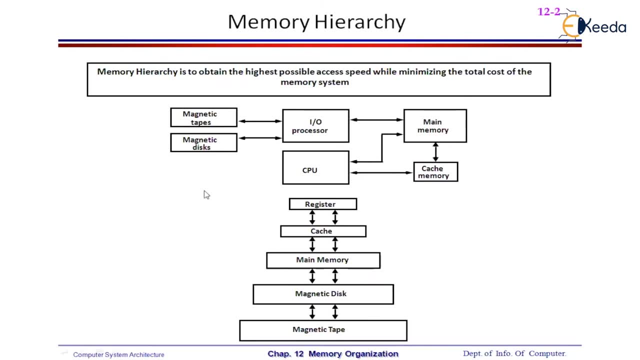 The program and data needed by the CPU resides in the main memory. Several times we discussed this. All other information stored in auxiliary memory, that is, in the secondary memory. okay, Now let us have a look at this memory hierarchy. We discussed about the main memory, which is the only memory that is available to the 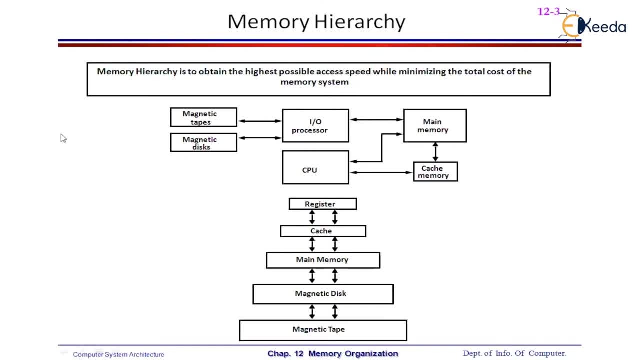 CPU In order to store all the programs which are not executed by the CPU currently will be dumped in the secondary memory. The programs that are being executed concurrently will get transferred to main memory. Hold on, Let us discuss something more important here. 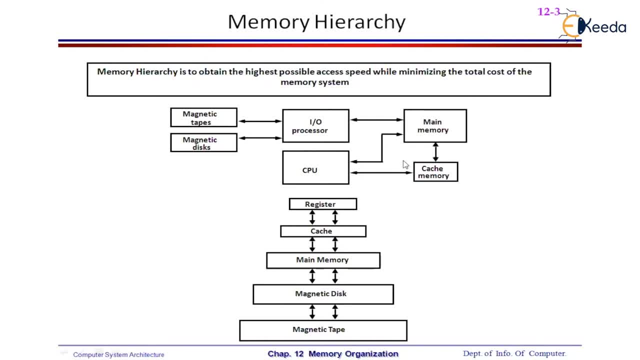 You can clearly see there is something on a cache memory. What is this cache memory all about? Why do we use this cache memory? Okay, Stay focused. When I ask you people, why do we require cache memory, You may tell me several answers. 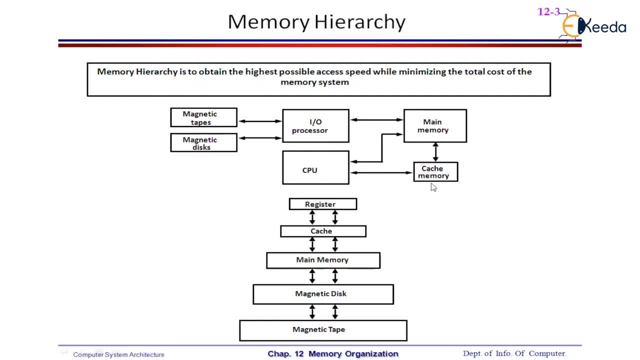 That is, cache memory is going to store the repeated data or anything that you may heard about the cache memory. But let me put it very clear to make you people understanding the purpose of the cache memory, The purpose of the implementation of the cache memory. 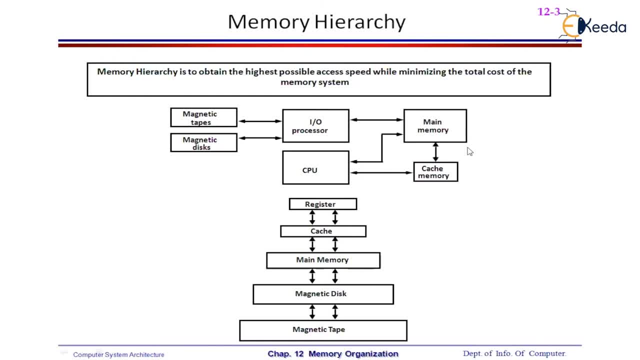 Okay, Now let us start. When we talk about the CPU, forget about everything, forget about all these things. Let us talk about the CPU. Okay, When you talk about the CPU, if I ask you a question, how to measure the speed of the CPU, how we can measure the speed of the CPU, let us have a look at it. 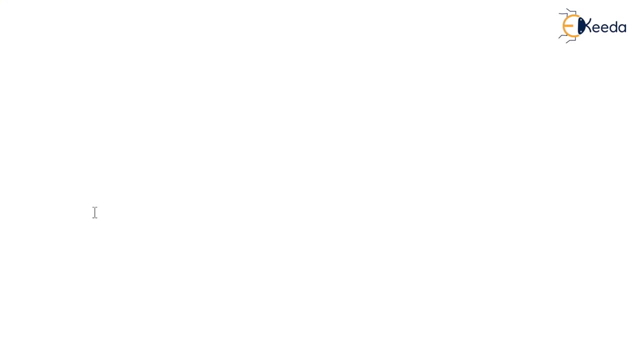 When it comes to a CPU, I will take a CPU. Okay, This is the CPU. Okay, This CPU is measured in gigahertz Right: 1 gigahertz, 2 gigahertz, 3 gigahertz and so on. 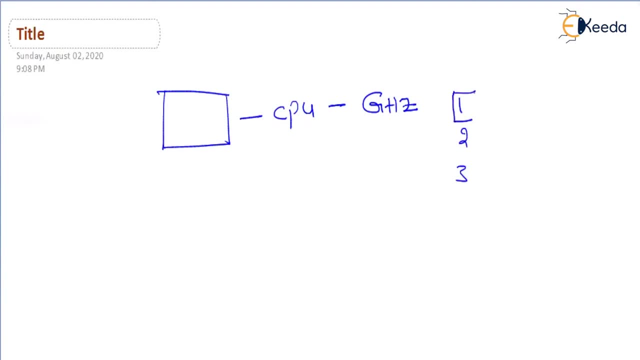 Now 1 gigahertz. I am taking the oldest processor, which is of 1 gigahertz capacity. What is 1 gigahertz capacity? 1 gigahertz is nothing but 1 byte, 10 power, 9.. 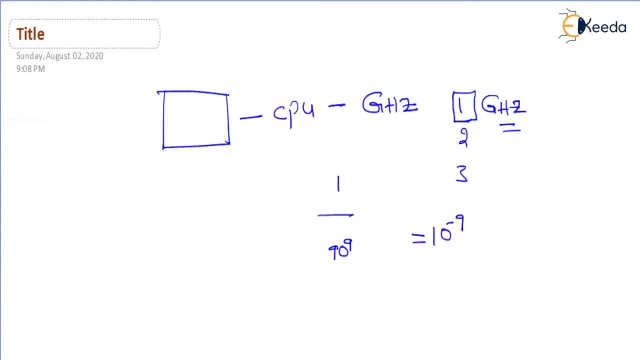 Okay, That is equal to 10 power minus 9.. If it is 10 power minus 9, there will be 9 zeros: 1, 2,, 3,, 4,, 5,, 6,, 7,, 8,, 9 zeros before a 1.. 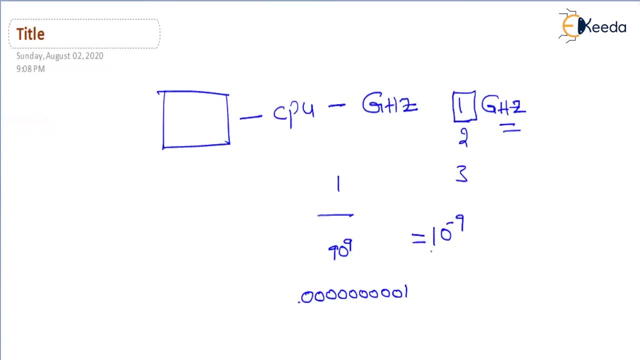 0.00090 and a 1. This is equal to 10 power minus 9.. Okay, Okay, A 1 gigahertz CPU- It is as fast as this one, which means that our 1 second will be divided into these many. 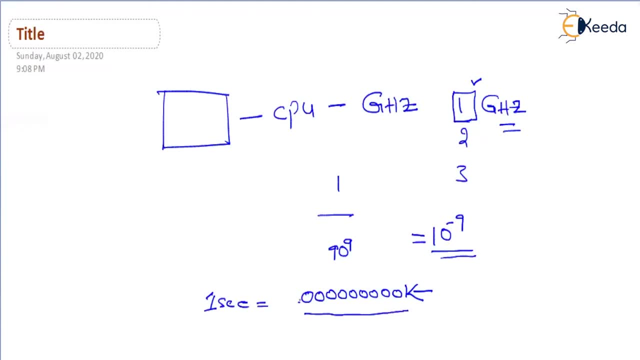 pieces, That is, after a decimal point, there are 9 zeros, followed by a 1.. Followed by a 1.. Okay, Which means that in 1 second, CPU will be able to perform these many pieces, And then the CPU will be able to perform these many tasks. 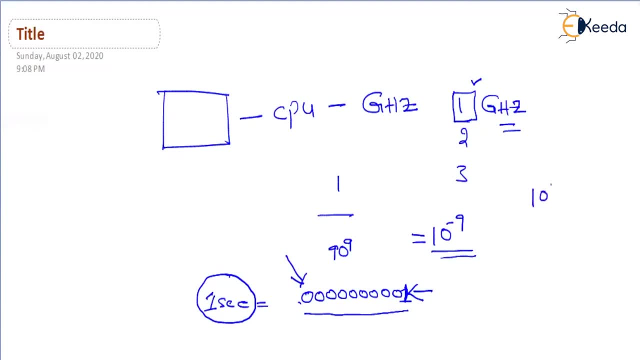 Okay, 10 power 9 tasks will be executed for 1 second. Okay, That is the speed level of the CPU: 10 power 9, it is crores, right, You know more than crores. 10 crores, 100 crores. 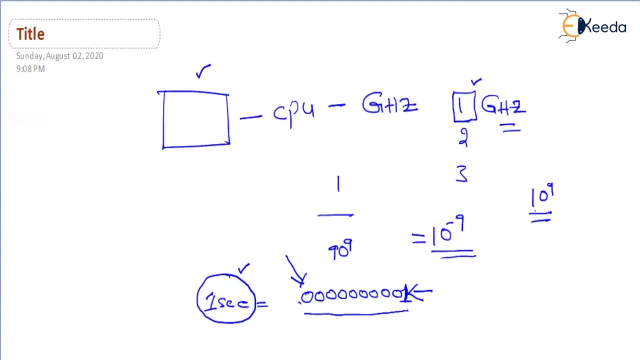 I mean 10 power 9 is very fast, in fact, Indeed, But still I am talking about 1 gigahertz processor, which is considered to be very slow in the current-day processor. The current-day CPU capacity, which is i3, is 2.66.. 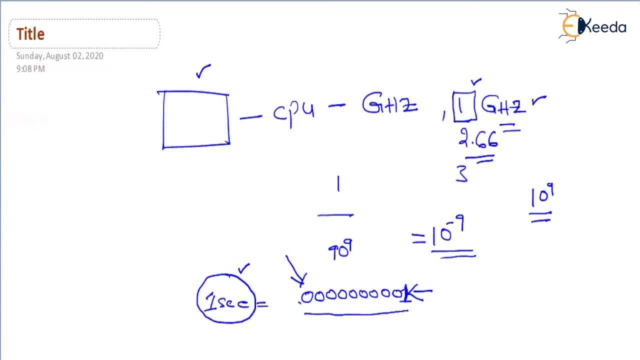 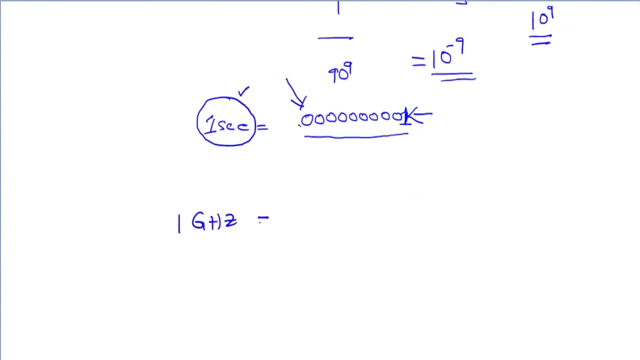 2.66 is way superior than 1 gigahertz CPU, right. So now I will, in order to get it simple, in order to make it simple now, we will understand just that 1 gigahertz processor is equal to 1 second will get divided into 1 crore clock cycles. 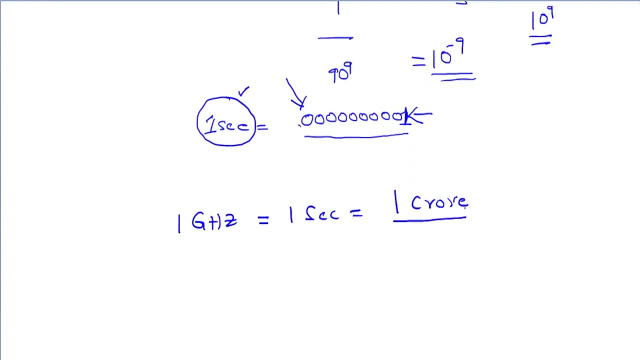 1 second will get divided into 1 crore clock cycles or nanoseconds, Whatever you call it. So a CPU will be able to perform 1 crore operations. Okay, CPU will be able to perform 1 crore operations in 1 second. 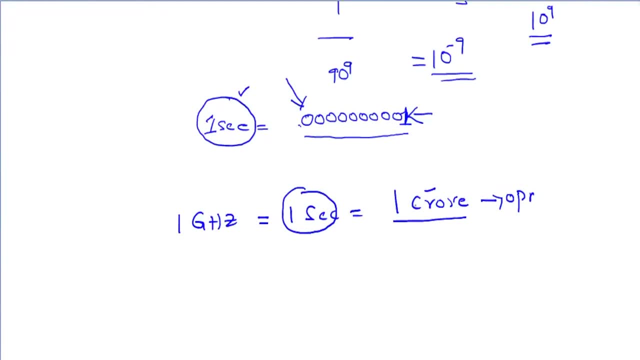 Of course it is not 1 crore. Let me tell you very frankly that 1 gigahertz is not equal to 1 crore. That is 10 power 9.. 1 by 10 power 9.. 1 by 10 power 9 is way beyond than 1 crore. 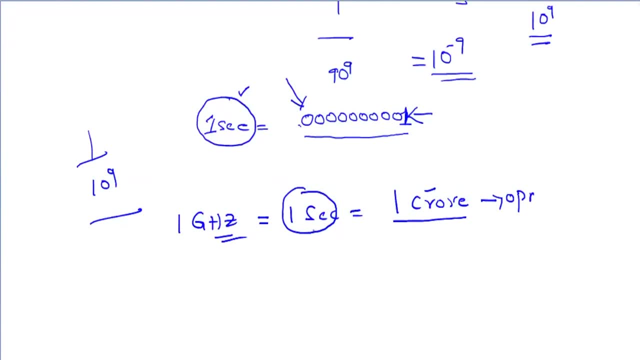 But in order to make it simple, we are thinking that 1 second 1 second will be divided into 1 crore clock cycles. Okay, Now let us understand. CPU is capable of executing 1 crore operations in 1 second for a 1 gigahertz CPU. 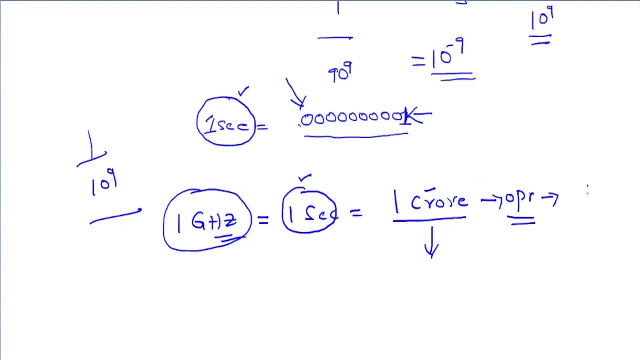 Okay, Now let us take that Each operation is an instruction. Each operation is an instruction, So provide, if we can provide it. If we can supply the instruction To the CPU, CPU will be able to execute 1 crore instructions in 1 second. 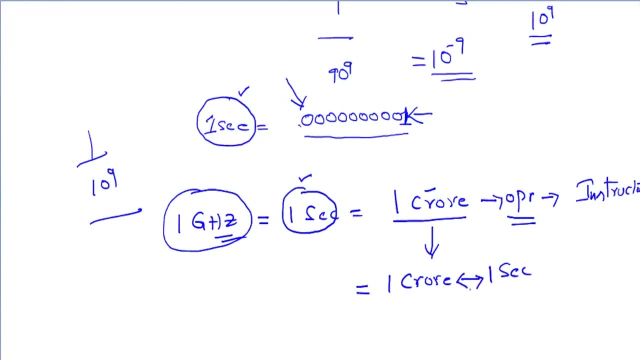 Did you get it? So this is the thing. CPU is very fast. That is how fast it is. A 1 gigahertz CPU may be a minimum. It will be able to execute 1 crore instructions in 1 second. 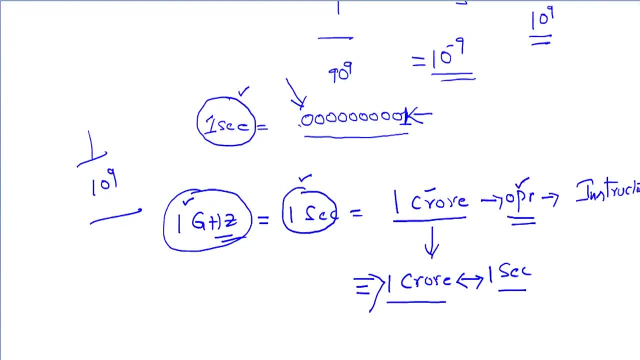 Because we are considering that each operation that is performed by the CPU is just nothing but an instruction execution. 1 crore instructions will get executed. You did it in 1 second, But hold on, There is something more to discuss here, Okay. 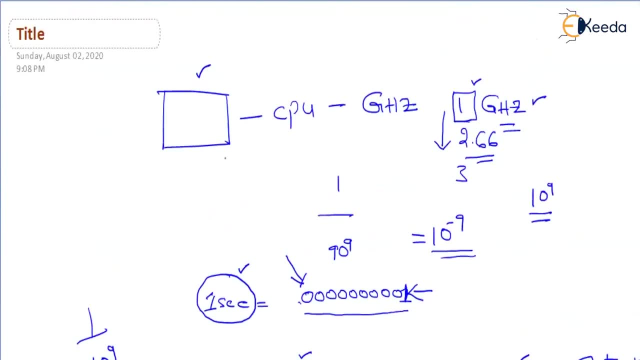 Now, of course, as I have a CPU, if somebody gives 1 crore instructions to the CPU, CPU will be able to execute 1 crore instructions in 1 second. But the problem is from where the instructions are given. instructions are fetched from main memory. 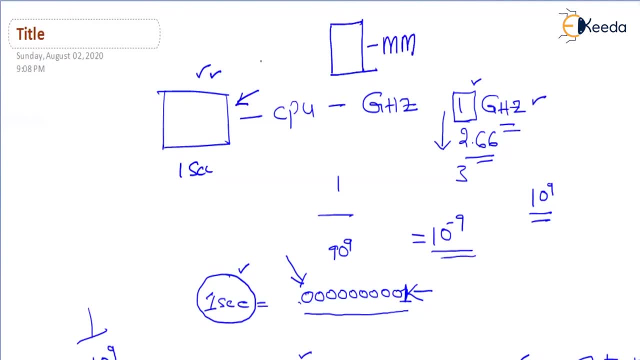 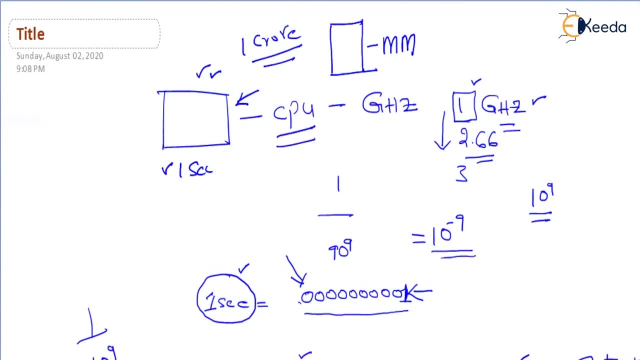 But the problem is, CPU is very fast, But the main memory, which is primarily a data supplier for the CPU is, on the other hand, is very slow. Okay, Main memory cannot supply, cannot reciprocate the request of the CPU. 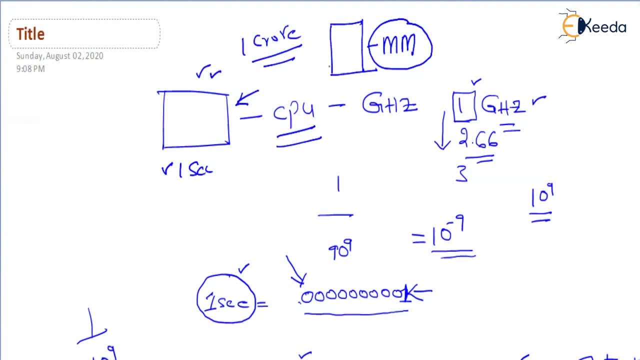 CPU will ask: Mr Main memory, if you can give me, give me one crore instructions per second. i am capable of executing all those instructions. but main memory will reply: mr cpu, you are the greatest person in the world. you are the fastest device in. 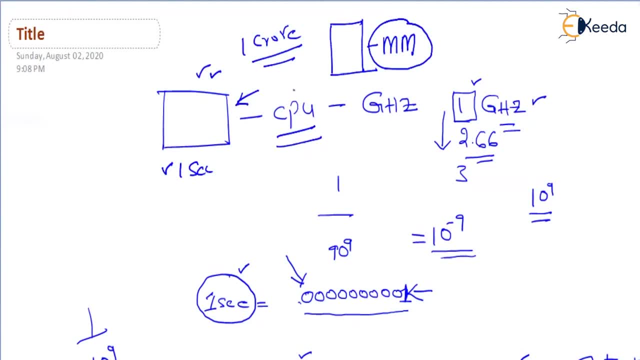 the world, but i cannot be as fast as you. okay, so finally, main memory will be able to supply only a few instructions. might not be matching to one crore, rather, main memory is giving just one lakh instructions. okay, now tell me how many instructions will be executed by the cpu. cpu is. 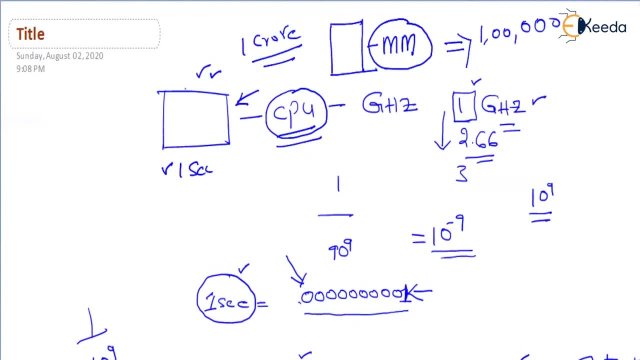 capable of executing many instructions, but it will be limited by the speed of the main memory. cpu is very faster, but, on the other hand, main memory is very slower. okay, finally, the total system speed is limited by the main memory speed, because the instructions and the data elements are to be